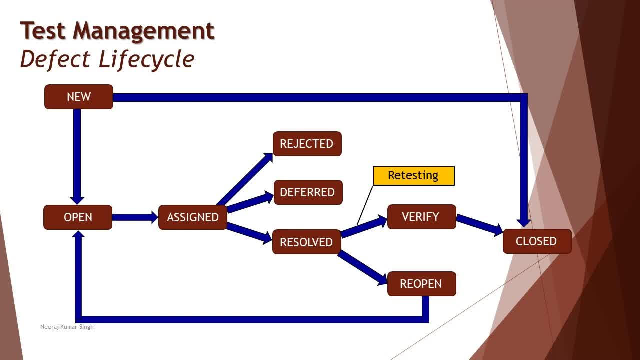 it at a different names, right, but again we are trying to starting with some kind of basic fundamentals of what exactly a typical defect life cycle- or quite often being called as bug life cycle- is all about. Now, here it is all about different status of a defect since it is reported. 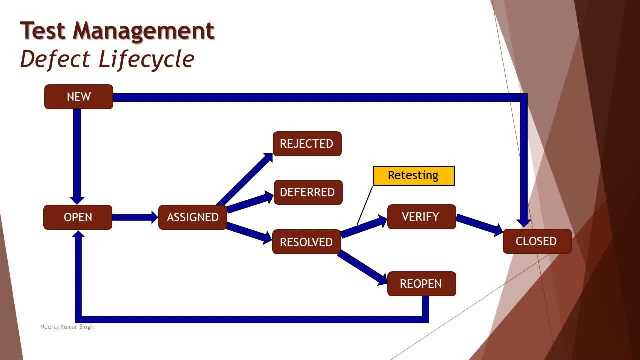 till the date it is resolved. Now, the journey of a defect has several status: to carry ahead and move from one particular person to another at different interval of time, and the most important thing here we will be talking about is what this journey is all about and how does it. 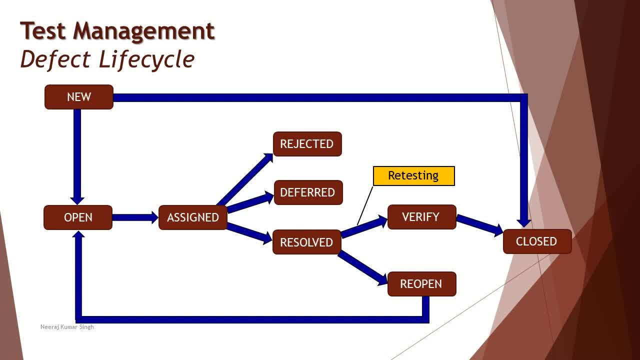 move from one particular person to another person within the organization. A journey of a defect starts with a status. new Now assume that a tester T1 was trying to test the system by executing a particular test case and unfortunately, or fortunately for our test engineers, the test failed. Now resulting this failure. the tester was supposed to log a defect. 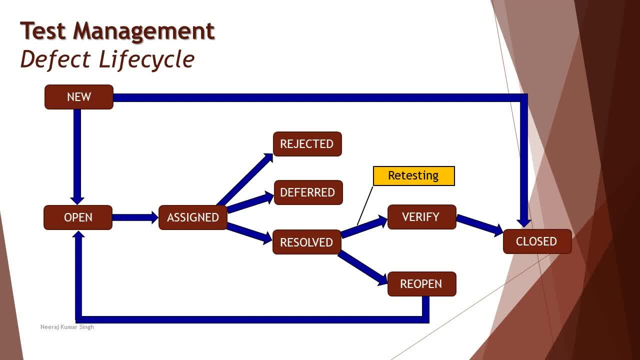 in the defect management system, which could be a tool as well- about the defect: what actually happened? Now, more importantly, here, a tester doesn't know what the defect actually happened to, that if that is exactly the defect or it's just a failed scenario. Now this could be a debate, as 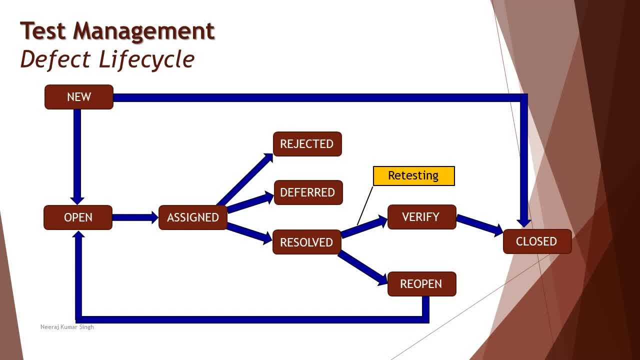 well to understand that a failure is always a defect. No, it's not necessary, because a failure could also be due to a tester misunderstanding, could be due to the compatibility issues, or could be a constraint in the environment as well. Now, initially, that's the reason. a defect is not always. 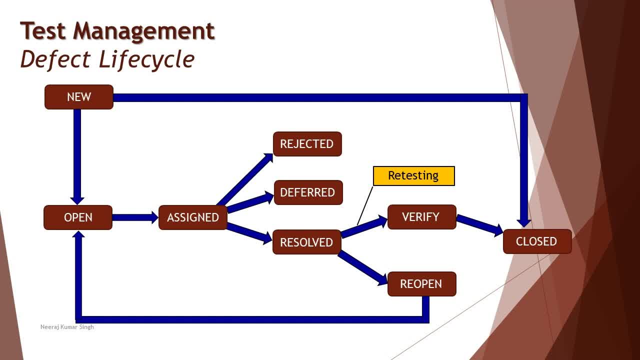 called as a defect but rather a failed scenario which is being logged. Now the status new will be given by the test engineer, who is logging the defect and in turn requesting someone superior in the testing team to review the defect. Now, at this point, a senior 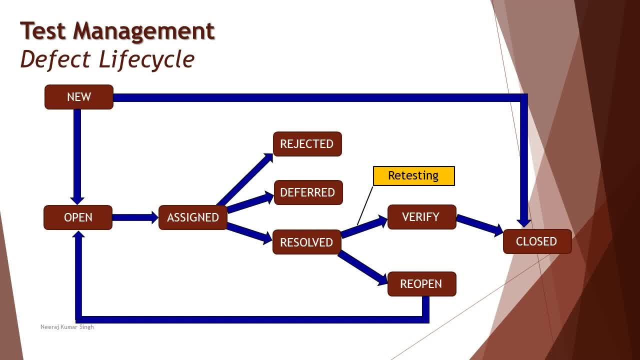 person in the organization- maybe your team lead or test manager will review your defects being reported and evaluate that if the defect is actually a defect, In case the defect is found to be valid, the test manager or the tester will review the defect and evaluate the defect. 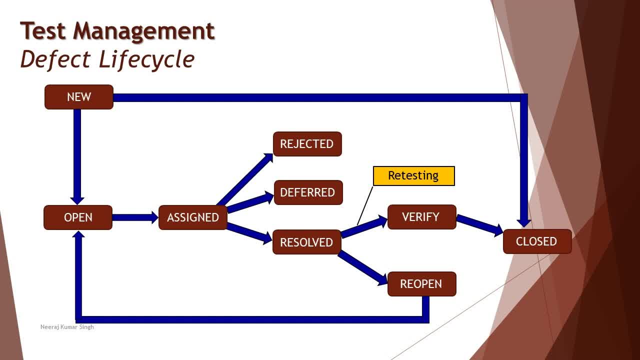 The senior person reviewing it will move the status from new to open. In case the defect is found to be a misunderstanding of the tester or probably another issue related to environment or compatibility, the defect will be moved back to the closed. Right from new status. it will be marked as: 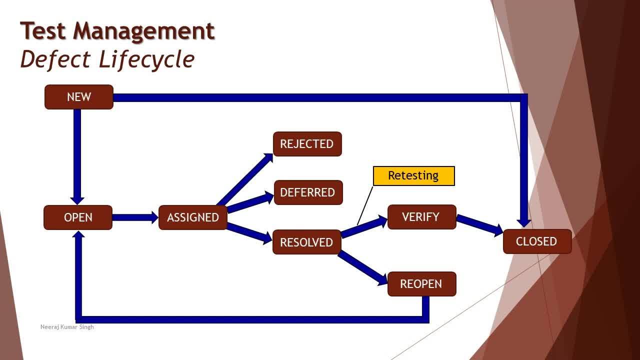 closed. that means this is not at all a defect where we have to waste a lot of our time. Once opened, it means that it's been handed over to the development team and the development manager has to look forward to understand the defect. Now the test manager will review the defect and evaluate the 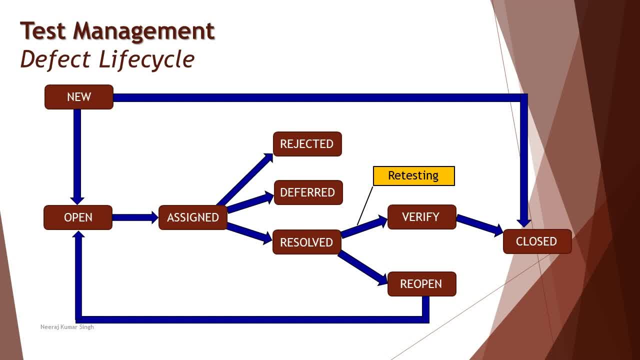 defect. The developer should also determine, when the defect is found, that which developer created the defect- as it's not a defect in the previous video- Because it will be easy for the developer to fix the issue, given that the person knows what is written and where. Right now, the development. 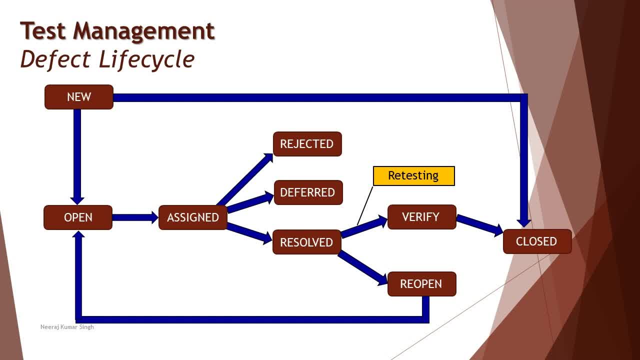 manager would identify the right developer and assign them. Now, this particular step could also be directly assigning to the developer, given that you are working in a gel, in a small team. So once it is assigned to the developer, the status of the defect should be changed from open to open. 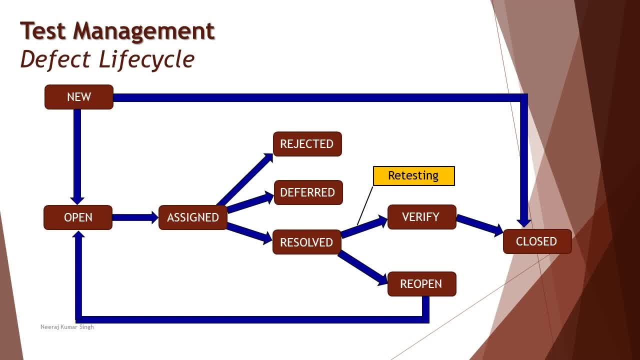 assigned, which always tells us that the defect is now with the developer and developer has to revert us back. Now, once assigned to a developer, developer has different options to provide you back on any of the defect which you report to them Now. these are the options. that is resolved. 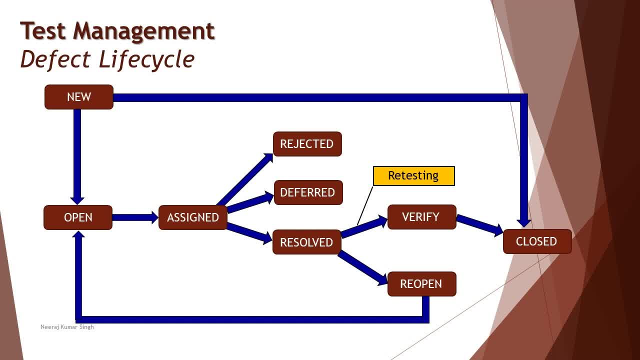 deferred or rejected, or maybe more Now resolved, is an option or status of a defect when the developer says: I have fixed the issues, you're good to go ahead and retest it. On the other hand, deferred as a status means that we agree and accept the defect, but we need more clarity to 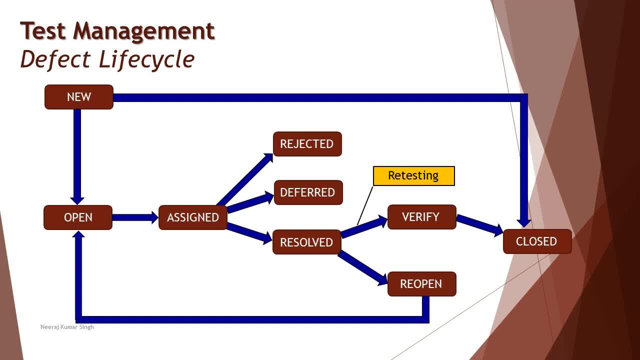 resolve the issue or there could be critical side effects of fixing the defect being reported. So we would need a business clarification or maybe the management approval to fix this issue and currently we are not fixing it. Deferred simply means that it will not be fixed right now. will. 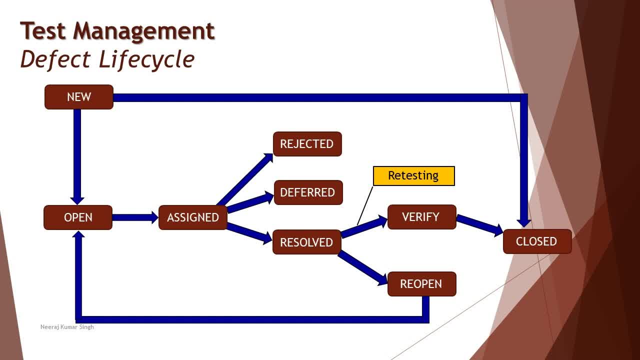 be fixed at a later point of time and could be, for any reason. On the other hand, rejected as a status for a defect simply means that the developers did not get it. That means it was working fine for the developer. Now this is another you know status for a big debate to understand why this could. 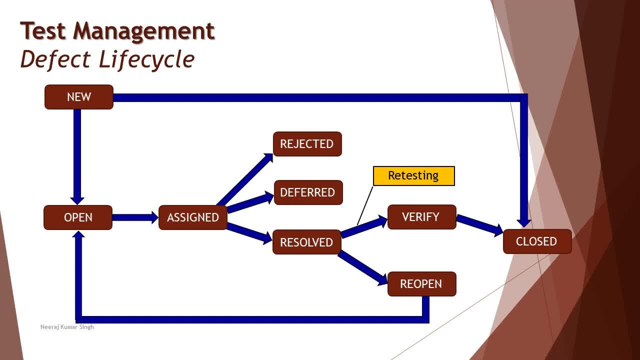 happen and what could be the reasons to say that a defect was not working in the development premises or instance or the environment? and it could also be due to the test data which you're trying or the environment you are using or, sometime, it could be even due to personal issues. 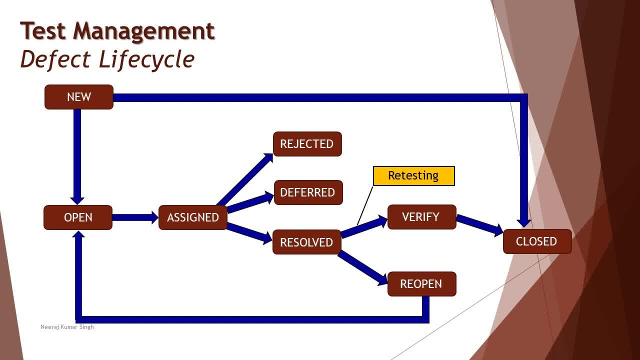 Right, Which will all come back to the same status, resolved at the end of the day, maybe sometime later. Once resolved, the defect has been passed on back to the test engineer who executed the test initially. Now the tester is required to rerun the same test, and that's what you call it as retesting. 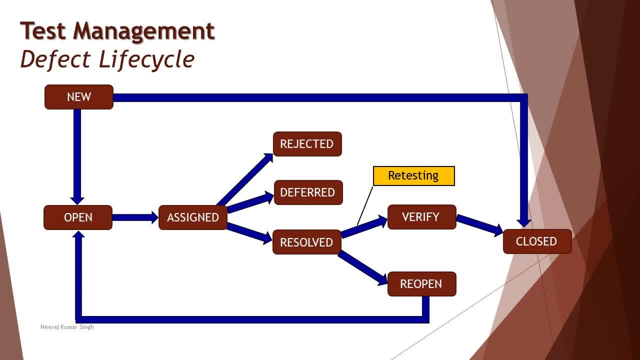 in our simple process. If retesting passes, that means the defect has been closed. but a tester, as he was not alone involved in opening a defect, will be requiring the assistance of the senior supervisor Or the manager who was who is going to review the defect whether it is actually closed or not. 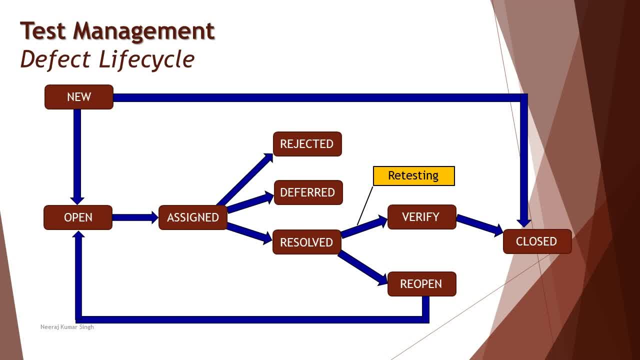 and verify it and close it Right. So tester, as he is not directly involved in opening the defect, same way will not be responsible for closing it directly In case the retesting does not pass. that means developer claims that he has resolved the issue, but when you performed retesting you 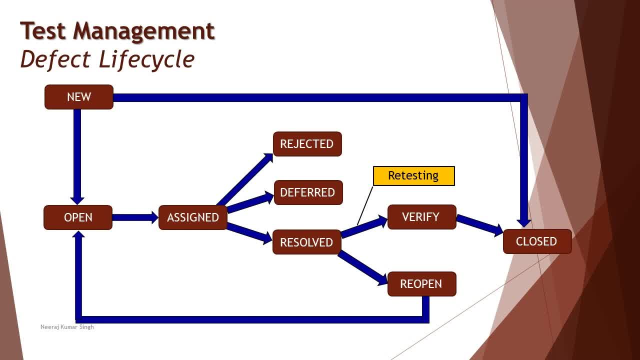 still found the defect. That means the defect is still not resolved. Of course developer took some efforts to close the defect, But maybe that step was not relevant enough to close the issue. Now you will reopen the issue here and the reopen means it goes back to the open state where it continues the same process as 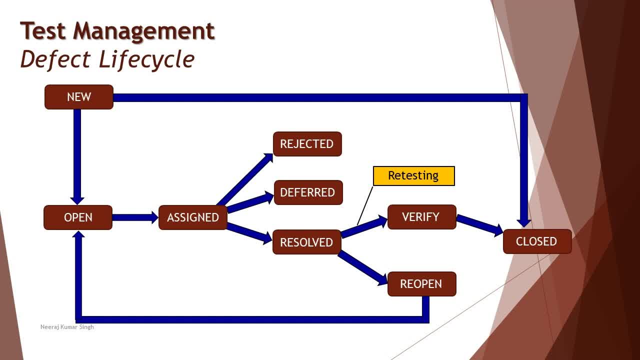 earlier till it gets resolved and closed. Now there could be some more options. for example, duplicate Now in case when you report a particular defect and you've reported another defect. but when we do the root cause analysis as a developer, you identify that the reason for both the defect and 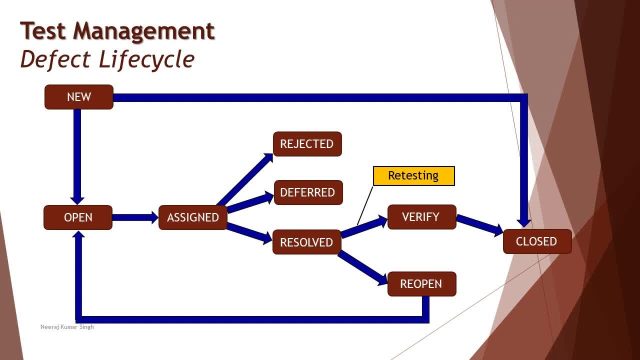 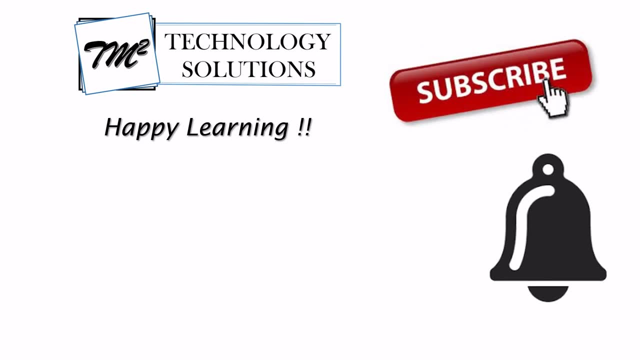 all the defects were same. Now you will mark one of them as resolved and the other one as duplicate. So again, developer have different other options and an organization can have several other things to talk about in your defect lifecycle. Right, That's all from this particular tutorial team. Should you have anything else, 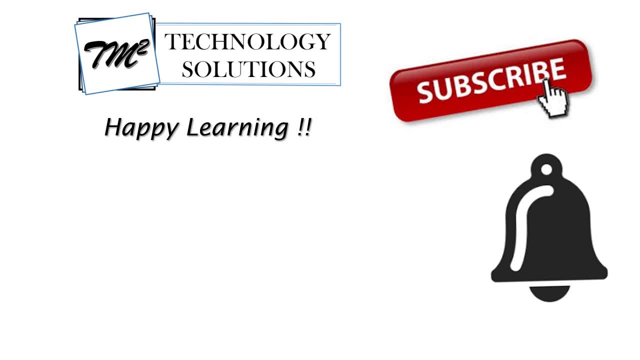 feel free to comment below. I'm always there to address your queries and answer them. well, Till then, keep learning, Keep exploring, Keep understanding the context. Thanks for watching the video team and happy learning.